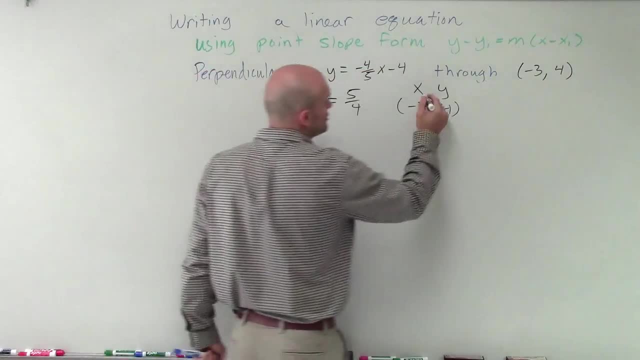 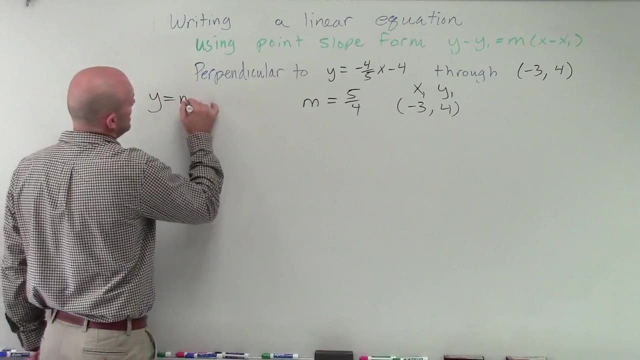 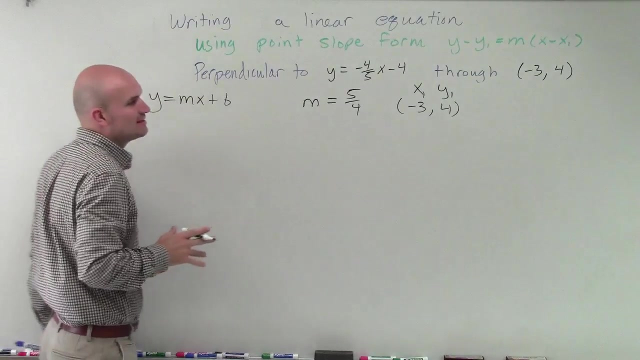 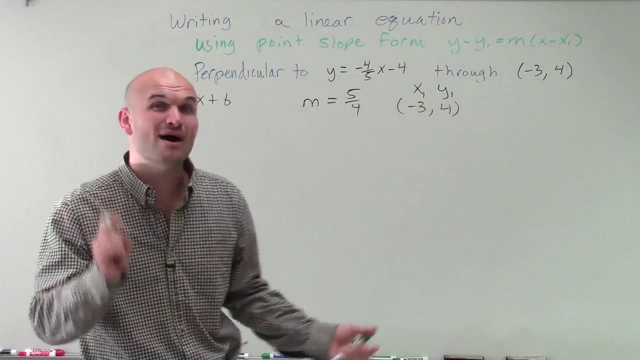 is that represents one specific point that we're going to use, And we want to make sure that we include the y and the x that represent all the points, because that's what we want to do. We want to find an equation of a line that's in slope-intercept form, where this y and the x- yeah, they represent any point, but they represent any point that can be on the line. So we just don't want to plug these in for our x and our y, because we want to make sure we write an equation that's going to represent all points. However, since we have a point, we can plug that in for our x1 and our y1 to make. 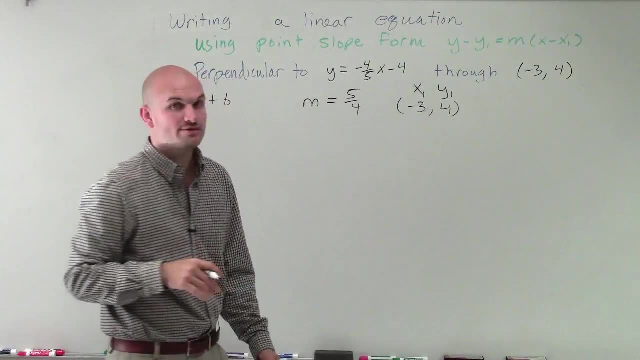 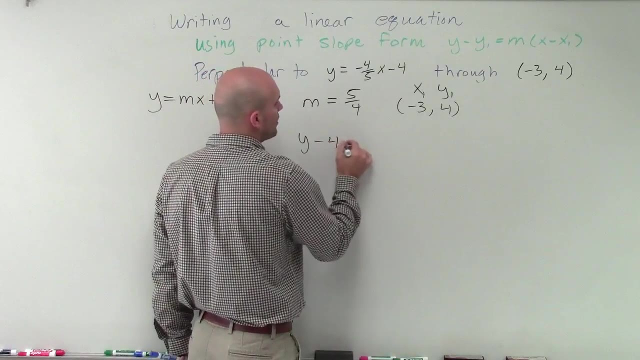 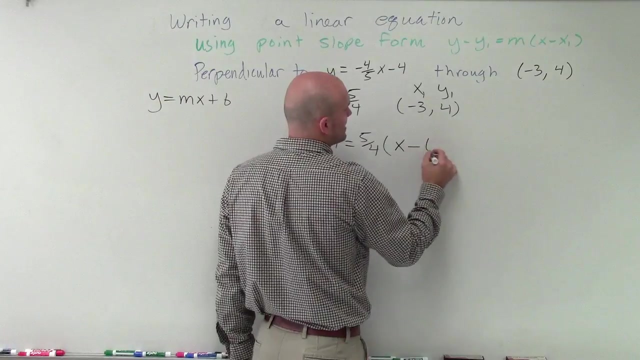 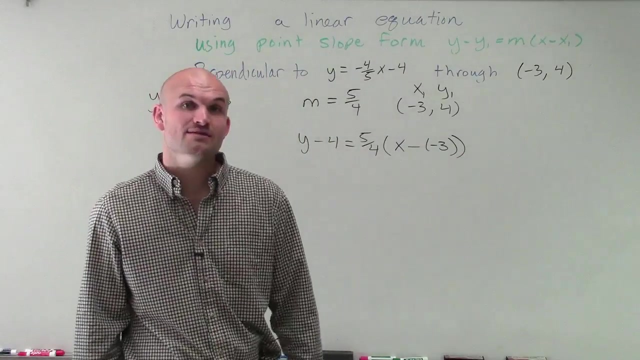 sure that we're finding the right equation, because we also know our slope is going to be 5 fourths. So what I'll do is let's plug in this information for what we have. So I have y minus y1, which is 4, equals m, which is 5 fourths times x minus a negative 3.. So we've got to make sure that we apply our parentheses to make sure that we don't mess up, and it's always x minus x1. Well, in this case, x1 is negative 3.. 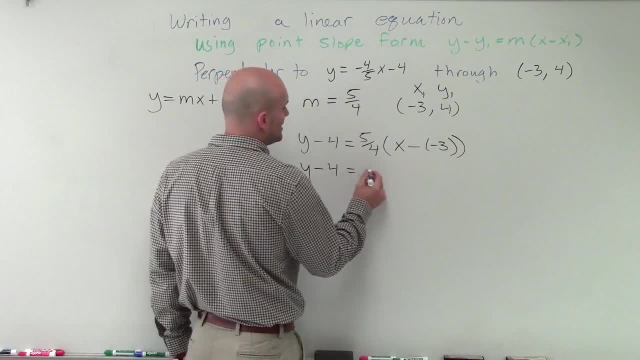 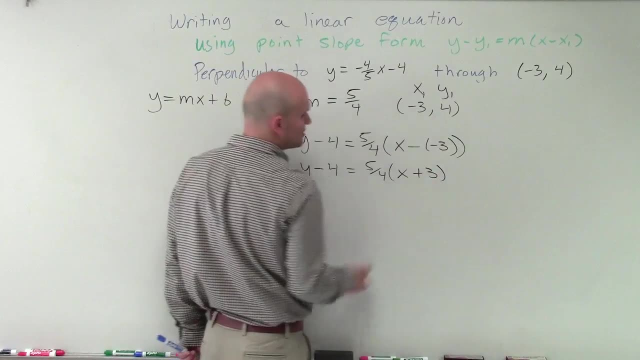 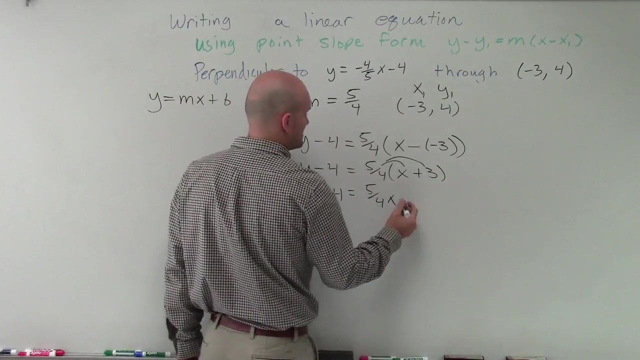 So I can't simplify the left side yet. so it's: y minus 4 equals 5 fourths. and I'll simplify this inside the parentheses. first, x minus a negative 3 is going to be x plus 3.. Now I can apply distributive property. so I have: y minus 4 equals 5 fourths, x plus 15 over 4.. 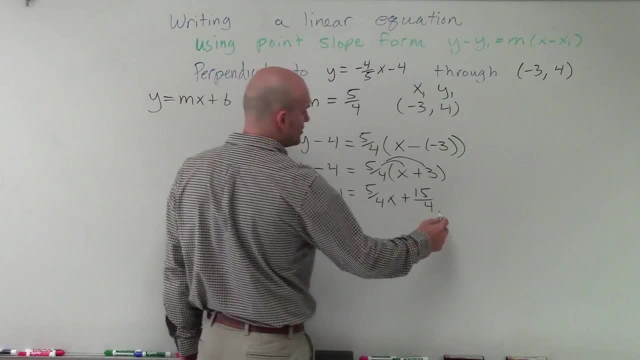 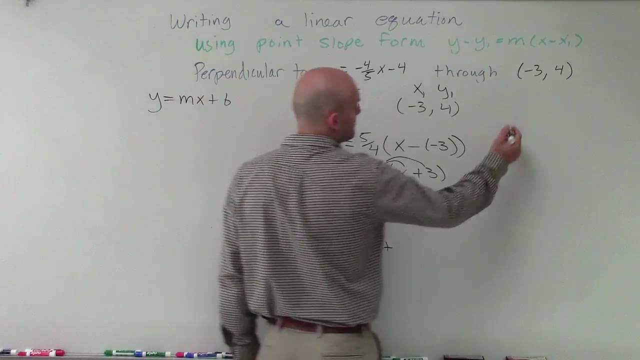 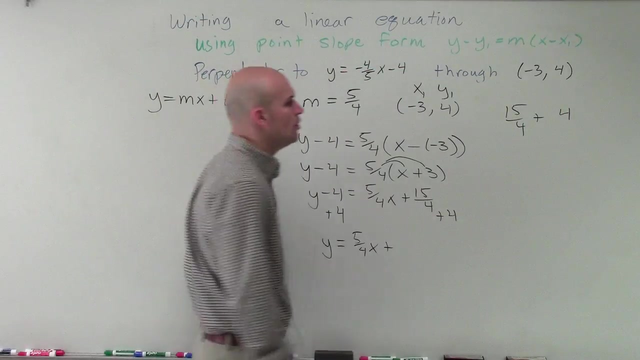 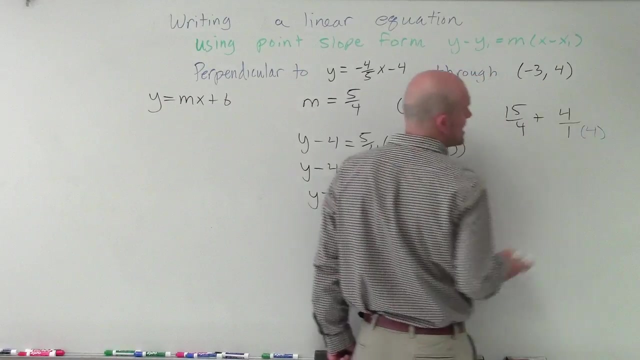 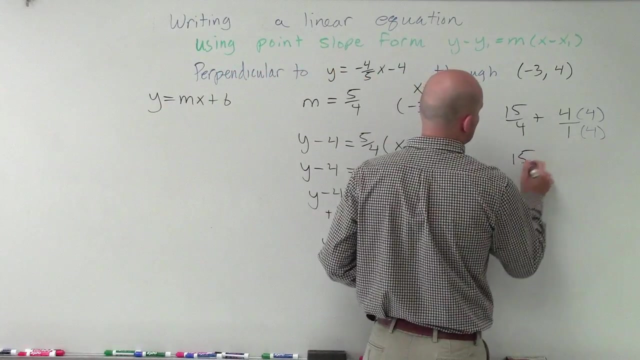 Then what I'm simply going to do is now add my 4 to both sides to isolate my y variable. So y equals a 5 fourths x plus 15 over 4 plus 4.. So to add a fraction to a whole number, I need to convert my whole number to a fraction. Then I need to make sure I use common denominators. So to get this to be common denominator, the common denominator is going to be 4.. I've got to make sure I multiply my fraction on the top and the bottom to keep equivalent of fractions. Therefore I have 15 over 4 plus 16 over 4.. Well, and that's going to produce me.